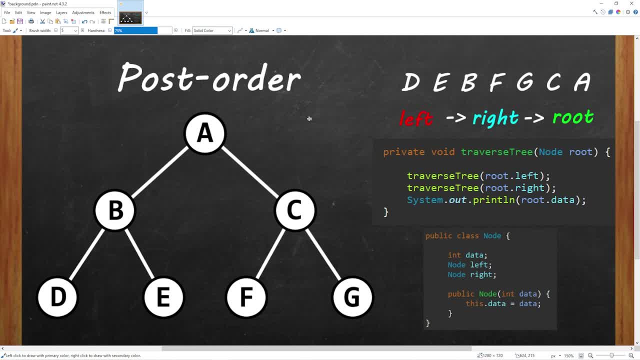 And here's post-order traversal. It's used to delete a tree from leaf to root and we follow this pattern: left, right, root. We will use recursion to visit the left children, then the right children, then the root. So A is our entry point. 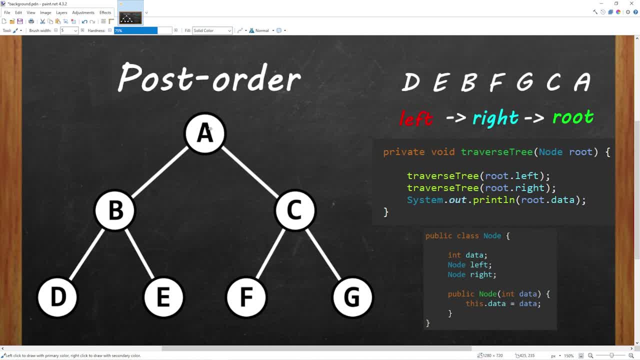 And here's our entry point. We are going as far left as we can, Go from A to B to D, Mark D as visited. Then we go right using recursion, Go from D to E, then root, Left right root. So we go back up, Go as far right as we can unless we encounter a left child. 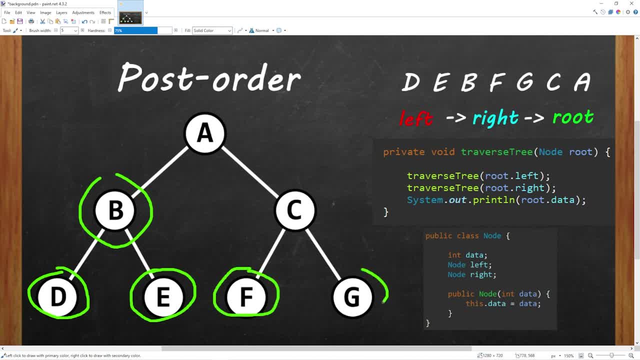 which we did. So we will mark F as visited, then G right root, Left right root, And all that's left is the root node. So that is post-order traversal. It's used to delete a tree from leaf. 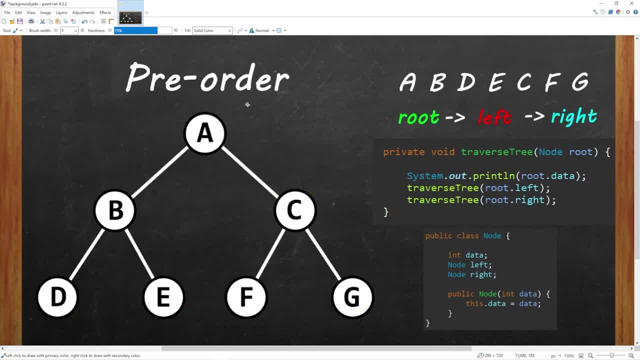 to root. And lastly, we have pre-order traversal. Pre-order traversal is used to create a copy of a tree. We visit any root nodes first, then left, then right. So we will mark A as visited our entry point, then visit the left child and we will continue to go left, then go right. So we 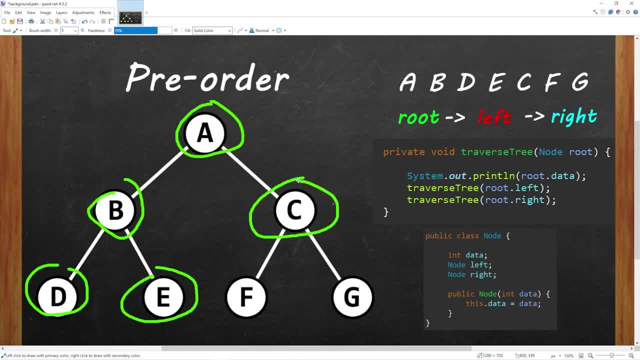 can't go left anymore. We're going to go right. So we can't go left anymore, We're going to go right. Mark the root as visited, then left, then right. This is used to create a copy of a tree. 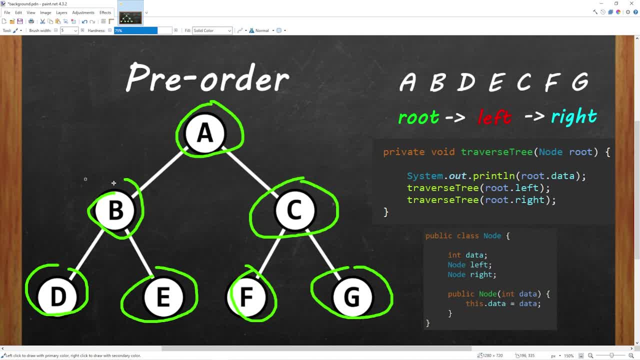 But in order to create a copy of a tree, you need to create a root node and a branch node to hold the leaves. So again, that's root left. We're still going left right. Root left right. A, B. 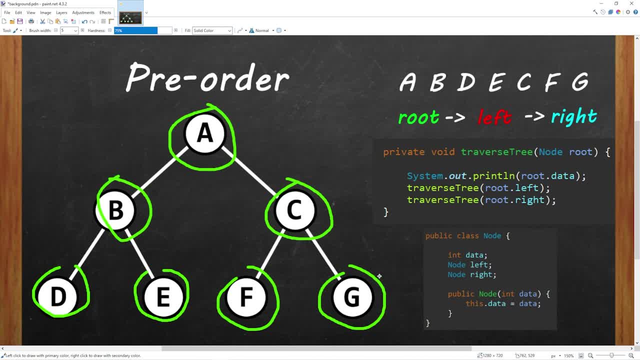 D, E, C, F, G. That is pre-order traversal. It's used to create a copy of a tree. Well, okay then everybody. That is a few ways in which we can traverse a tree. Like I said, normally we don't have random access, So the entry point is the. 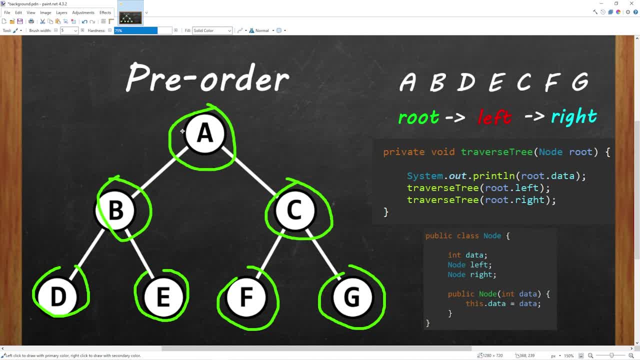 root node And you can either follow an in-order, post-order or pre-order traversal, depending on what you need to do with this tree. So that's tree traversal in computer science. If you liked this video, please be sure to give it a thumbs up, leave a random comment down below and subscribe.